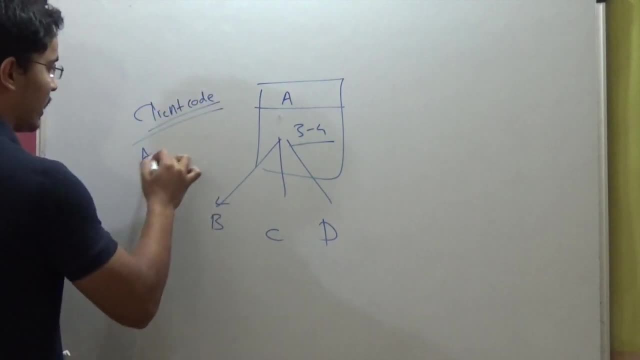 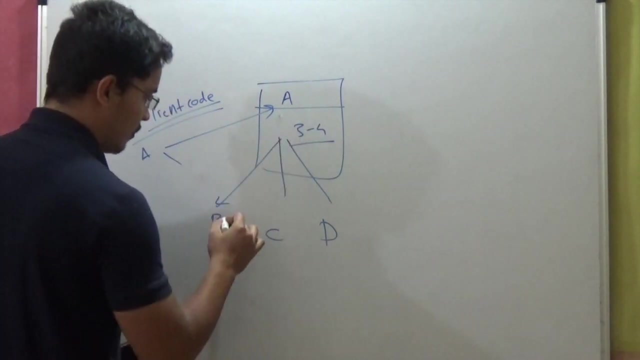 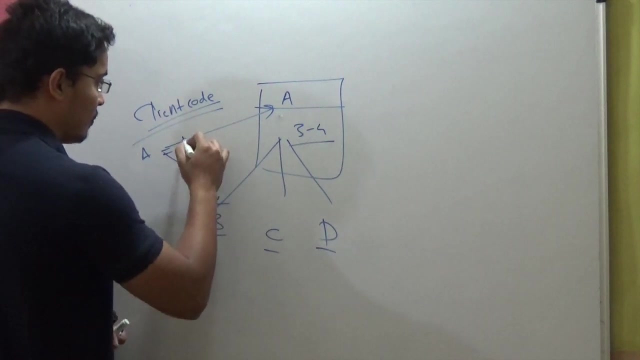 So if client code we are trying to create object of A, we have two approaches: One based on certain condition: it will be composed of either B, C, D or all of them. So that complex logic of first creating B, then C, then D, then composing them together to create A. 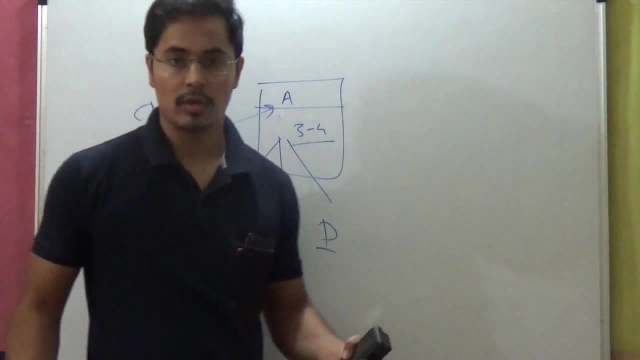 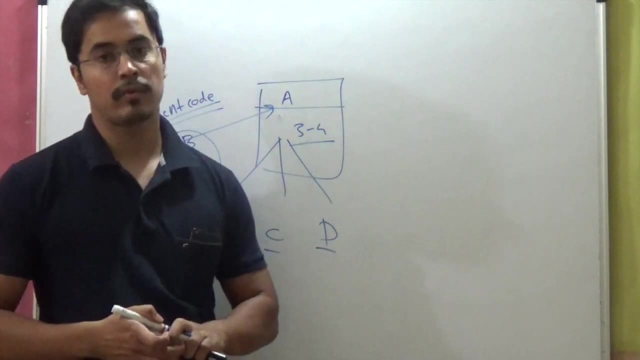 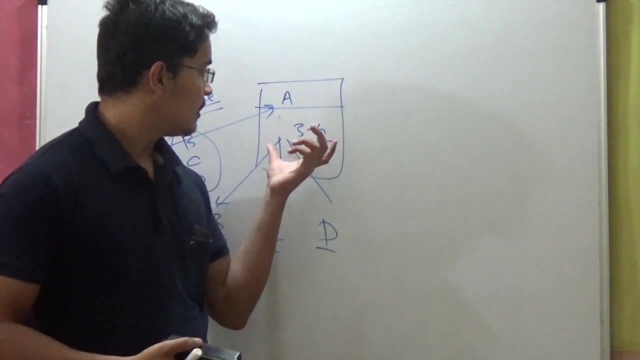 and then, using A, could be put in the client code, or we can extract it out into another component. So this is the component called as builder. So this is precisely what we are going to do: We are going to create a builder which will take care of that complex logic of creating the composite, complex object and isolate that logic from the client side. 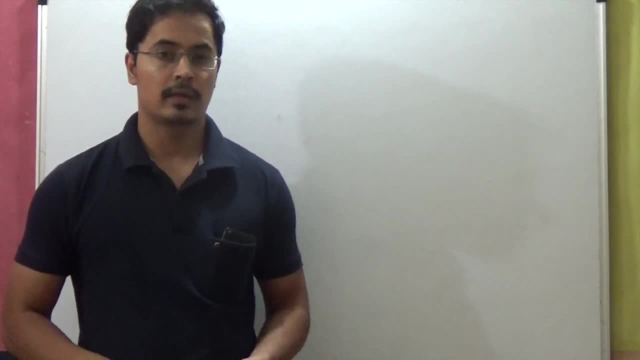 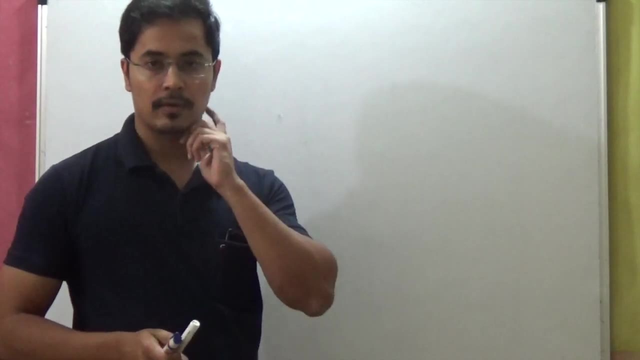 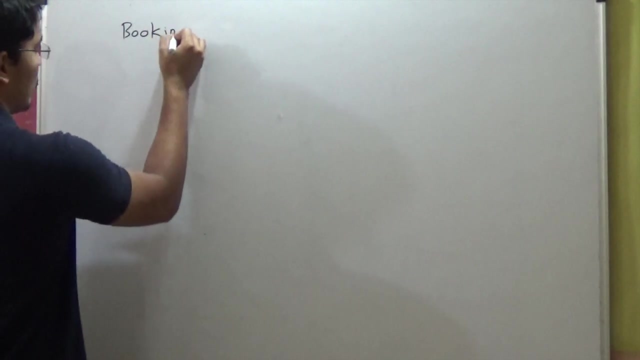 So let's do that. Let's take an example from our tennis court booking application. In the video of decorator pattern, we gave ourselves functionality of doing different kinds of booking. That is, it could be a simple booking. Booking was of type individual court booking- coaching session. 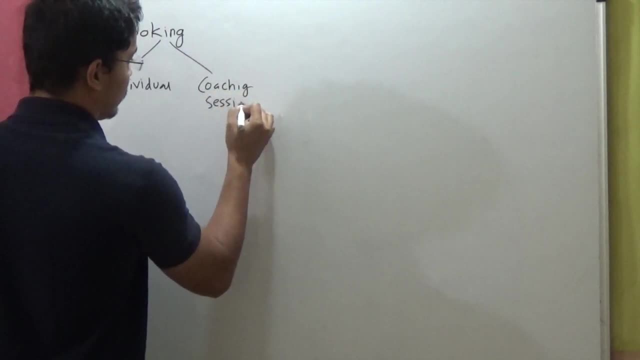 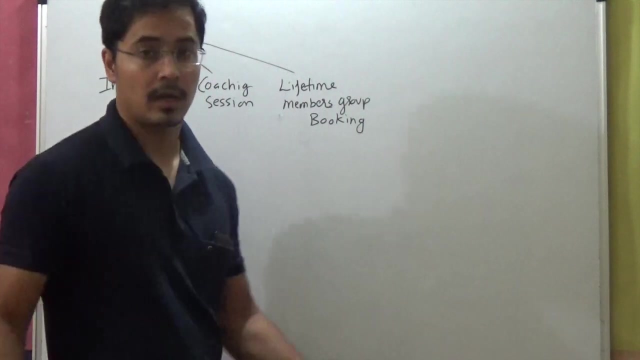 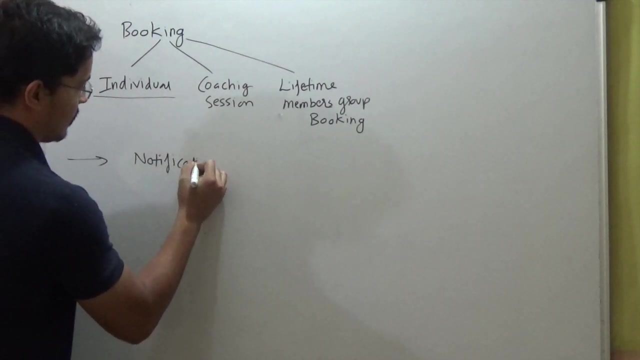 So you could have coaching session. We also had lifetime members group booking. This is one more type of booking that we are allowing. In the scenario of all these three bookings, we want to send notifications- Notifications about the details of the booking. 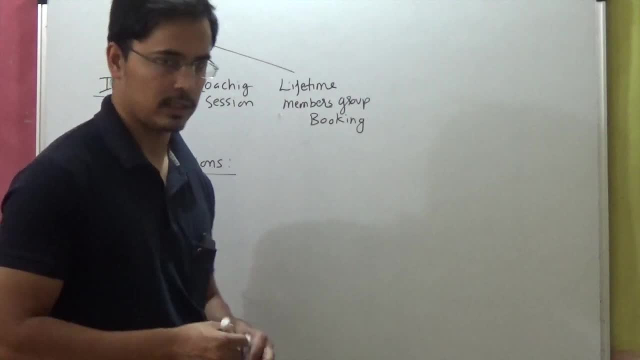 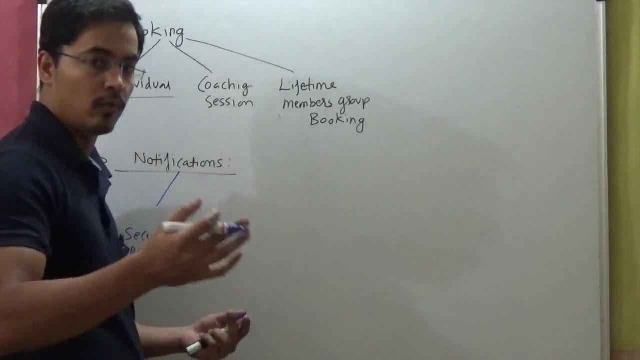 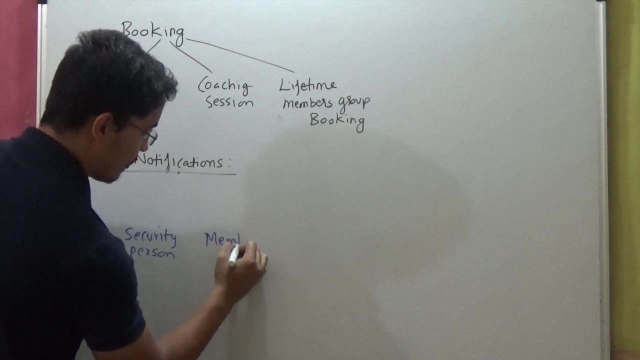 To whom can we send this notification? So we can send this notification to the security person present on the court Who can permit or not permit the entry of the members. Member itself who have done the booking Members. Then we have coach. 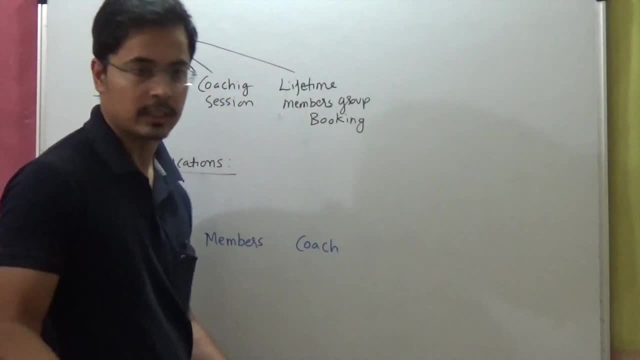 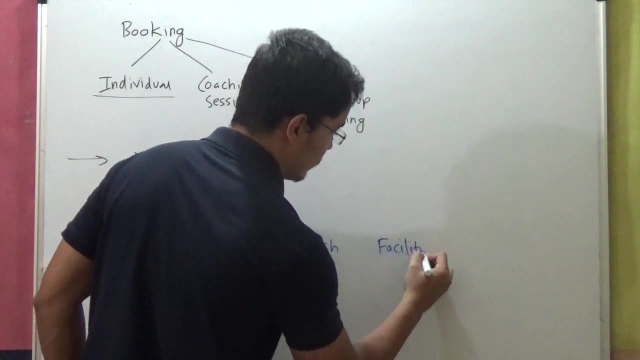 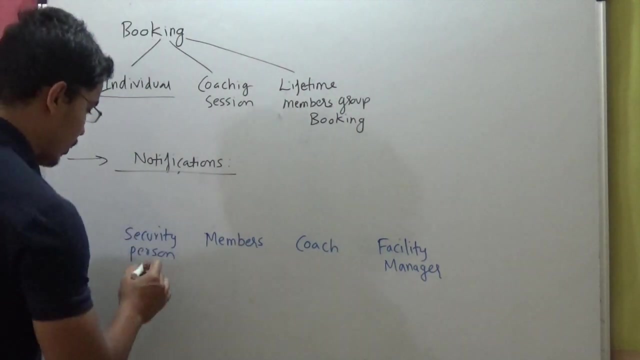 In case you have booked coaching session, we will have to notify coach, And then we have, let's say, faculty, We will say facility manager. Now, in case of individual booking by members, we only need to send notification to security person and member itself. 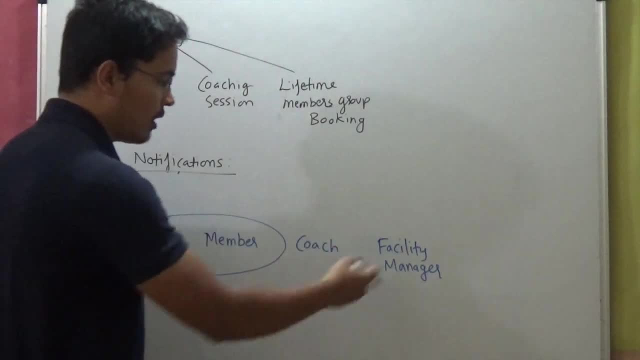 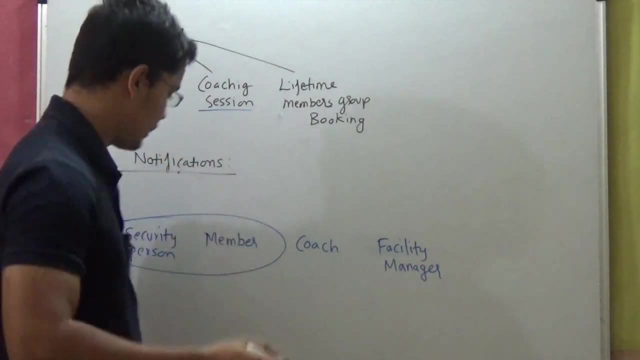 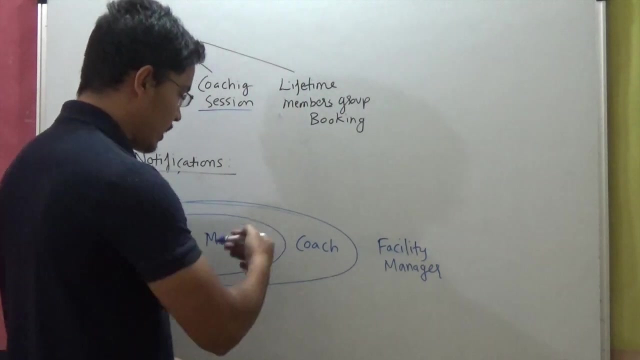 Security person and member, Because coach is not involved and facility manager doesn't need to be bothered about this. In case of coaching session, we need to notify security person, member and coach- All three of them Right- Because coach is going to conduct the session. 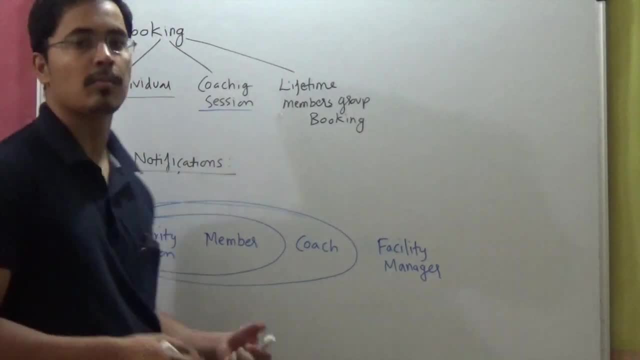 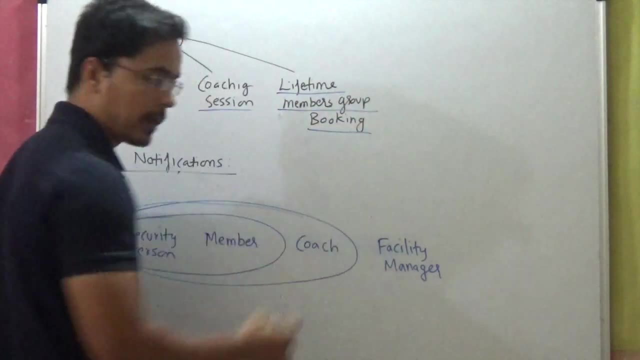 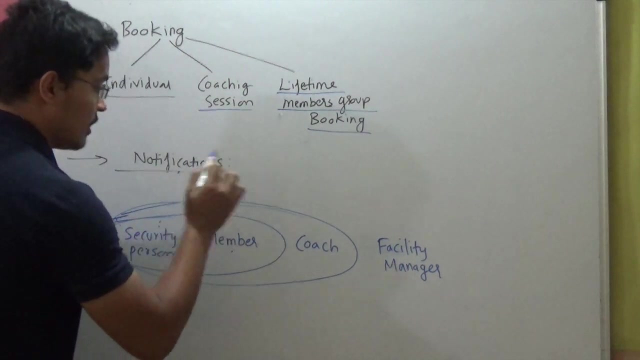 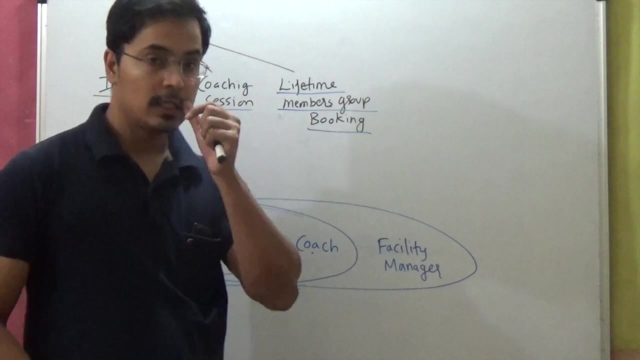 Member is going to attend the session And security person must know session is happening between coach and member. In case of lifetime members group booking, we want to inform or notify security person, Obviously members, coach and facility manager also, Because in that case these customers are special customers. 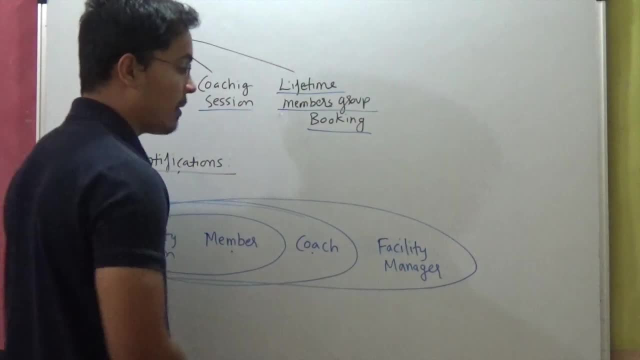 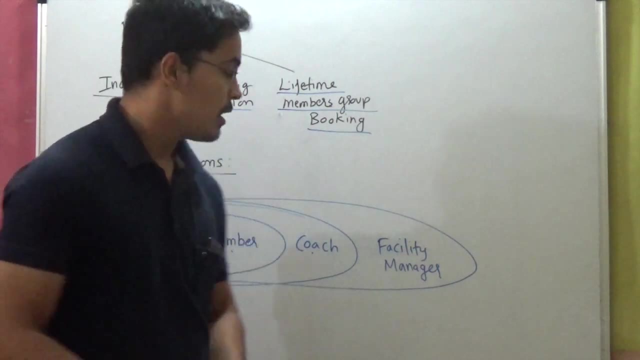 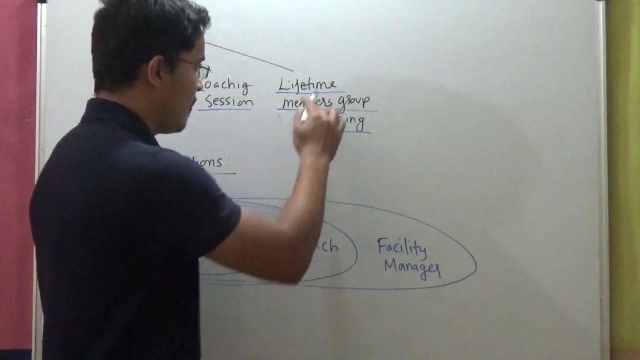 For the tennis complex. So the facility manager must be kept in loop That lifetime members are having a group session on certain so and so day Coach, because in this kind of booking we have decided that we will make sure that one coach is available for the lifetime members group booking. 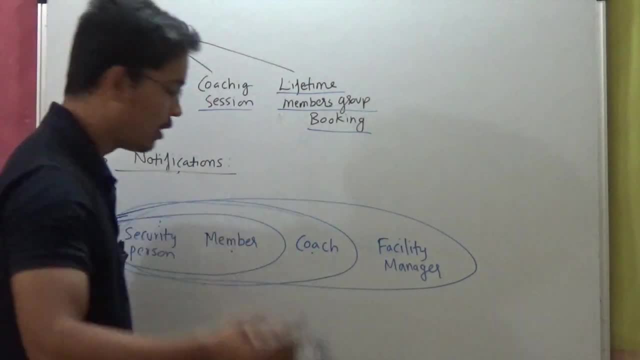 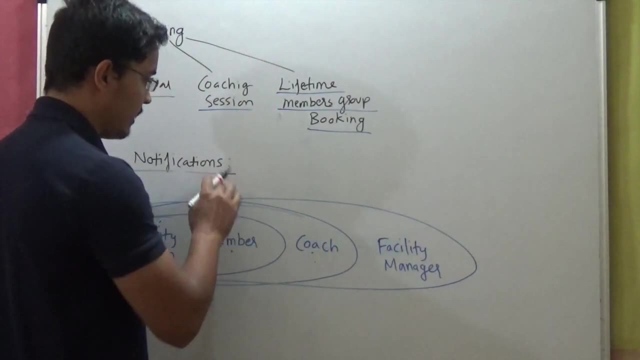 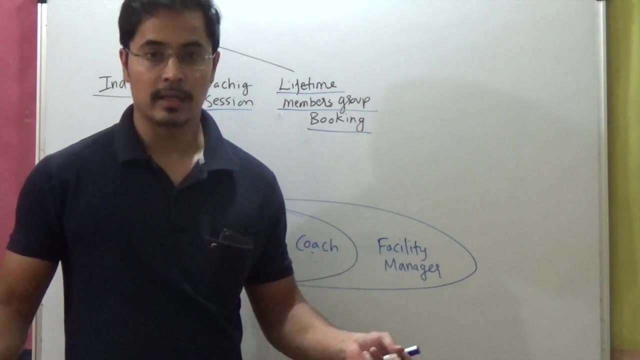 In case they need him, Right. So coach has to be kept in loop, Members, obviously, and security person. So you see, creation of this notification. object: Right Can involve different stakeholders based on the type of booking. We can further complicate this and it will get complicated. 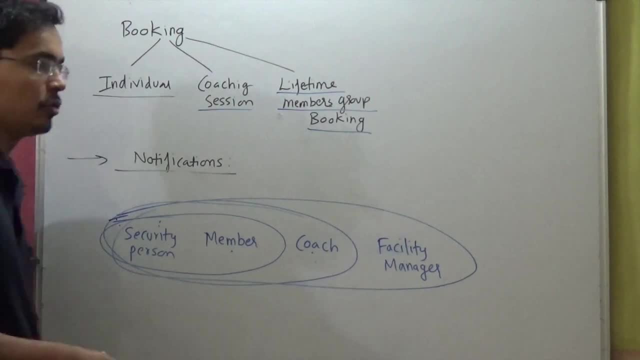 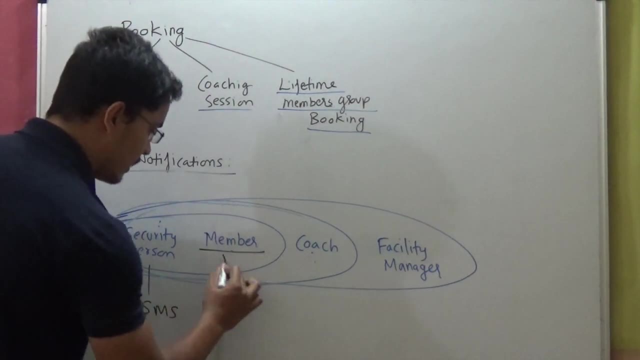 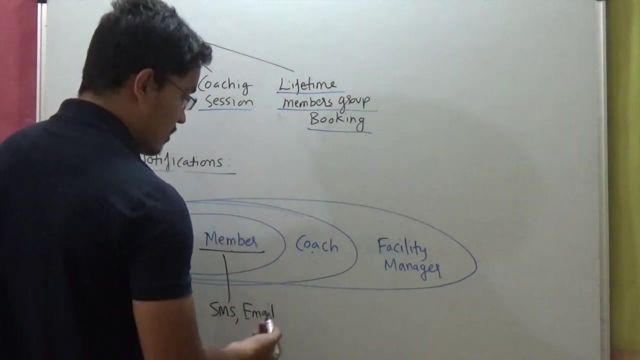 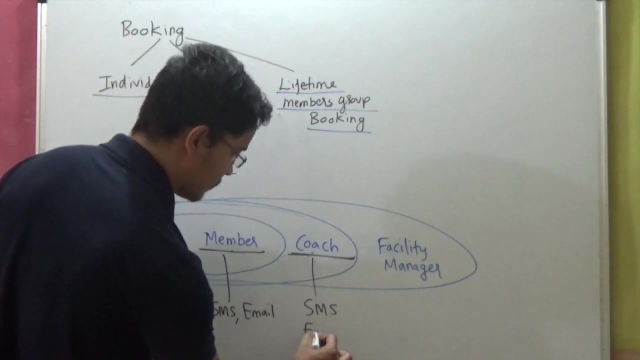 For example, security person do not use emails usually, So they will need SMS notification. Members will need SMS and email both. Right Coach will need SMS, for sure, And let's say email too, Whereas facility manager will only need email notification. 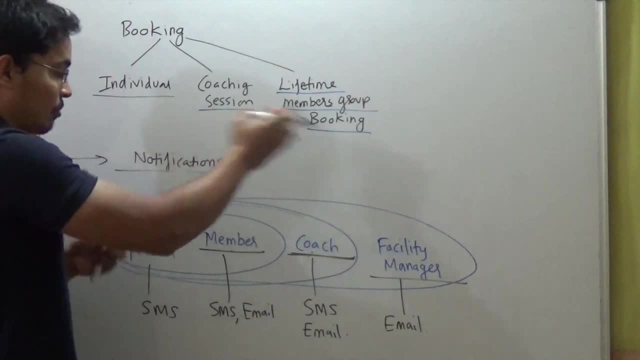 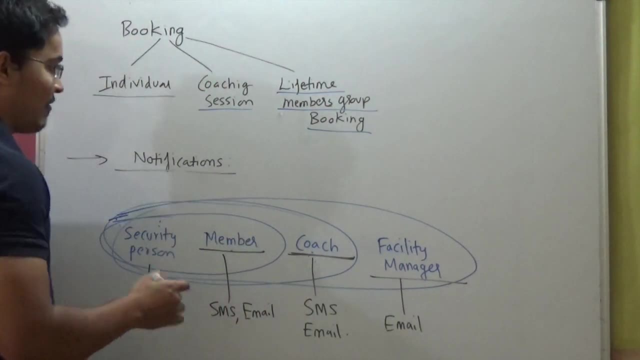 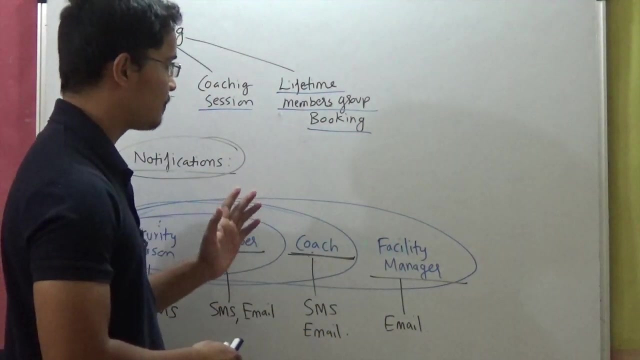 First, stakeholders are different for different kinds of booking, And then mechanisms are also different. So safe to say that after you create booking any of this kind, While creating the notification you have lot of things to consider. So, in this case, the way I am going to design this problem, 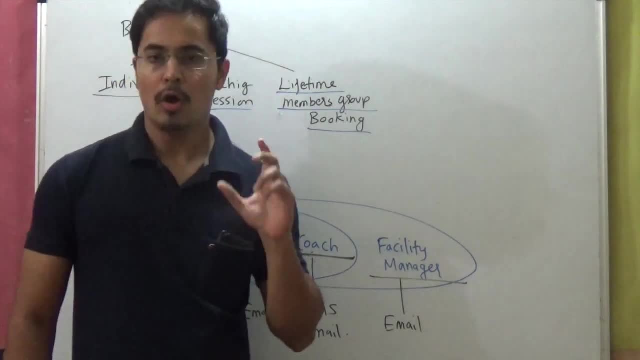 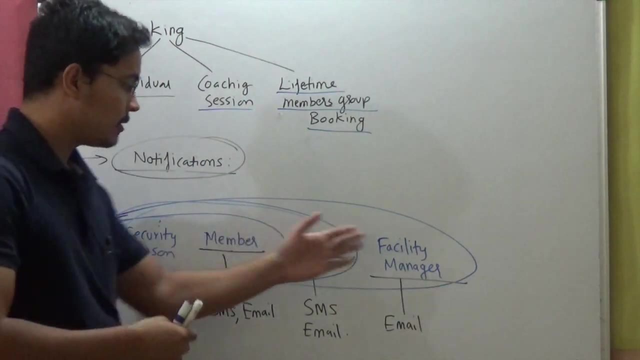 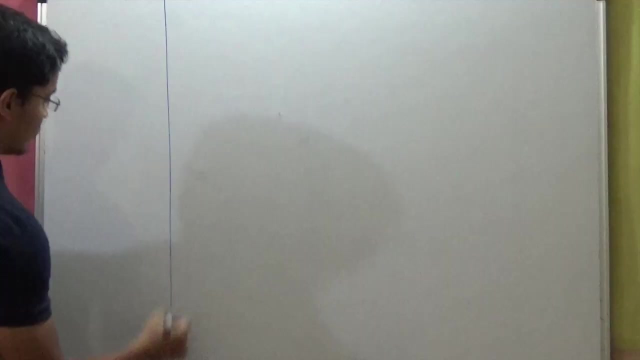 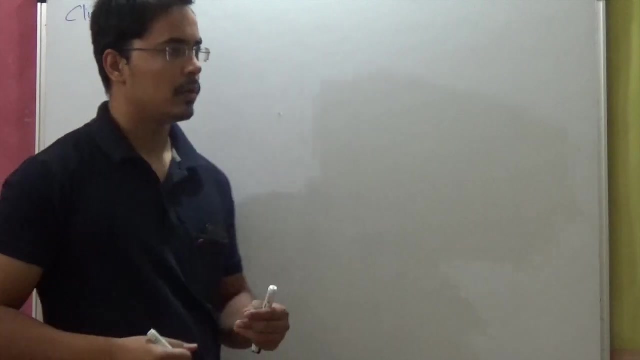 Is that my notification object will be a composite object Right, And then, based on the conditions, I will choose the correct composition. Let us see how can we use builder pattern to solve this problem. So this is my client code. Client code is nothing but the place where we are going to need to send the notification. 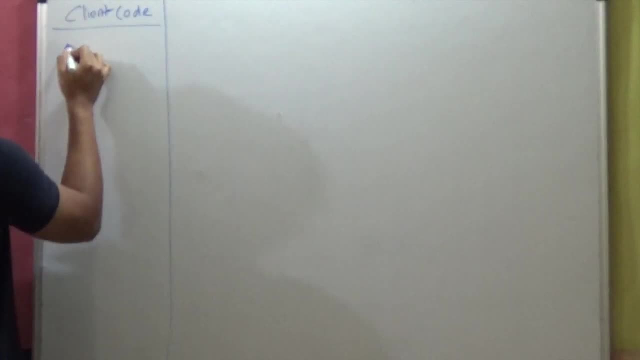 So it will usually happen After, let's say, we create a booking object, Booking object of some kind, Right, And we say bsave- Right. So we have created booking, Right Now we need to send notifications regarding about this booking. 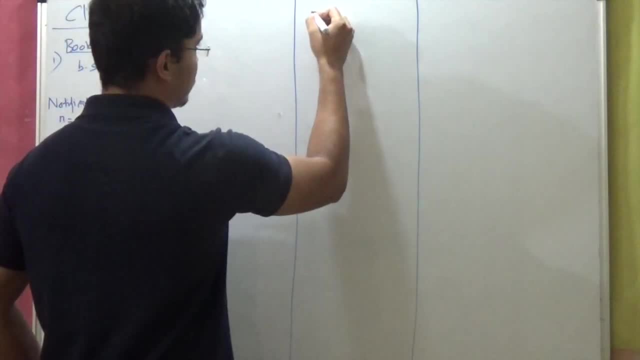 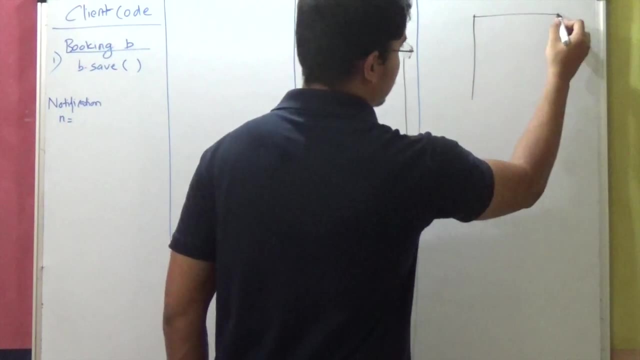 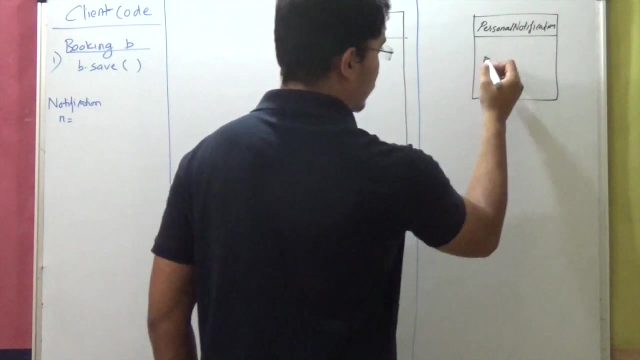 My notification class is going to be something like this. Prior to that, I will write my lowest level object, That is, I have an abstract class called as personal notification Right. It will have a method called as send notification. This is the abstract method. 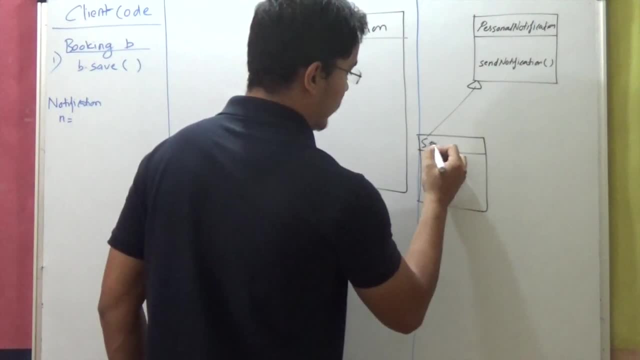 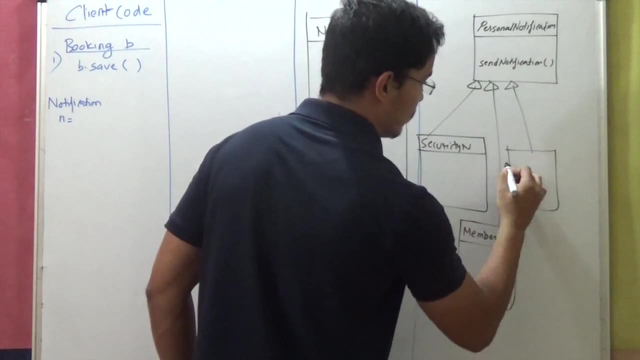 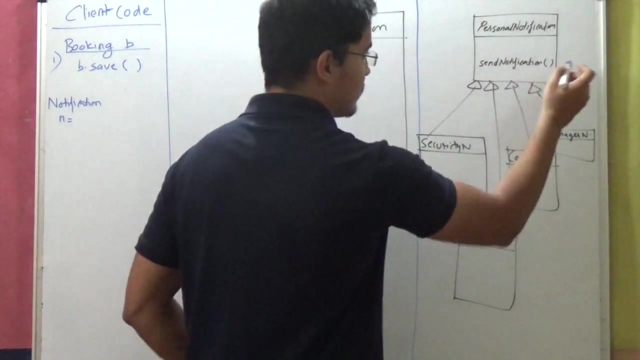 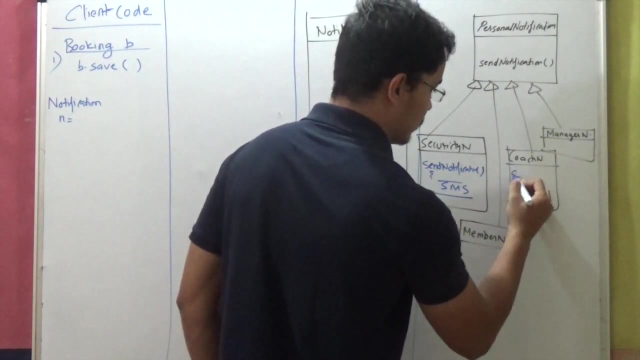 I am deriving four concrete classes from this: Security notification: Member notification, Coach notification, Manager notification Right. They all will have to implement this send notification method. So here security will only send the SMS Coach send notification. It will have SMS plus email. 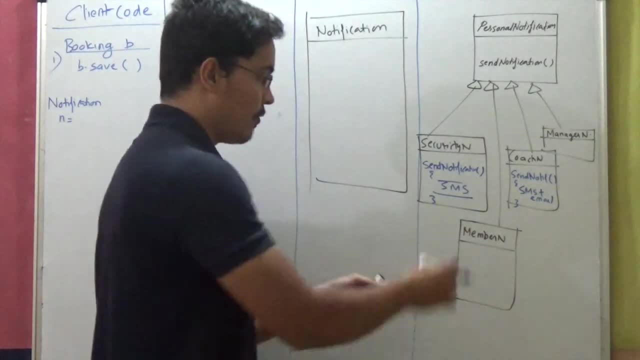 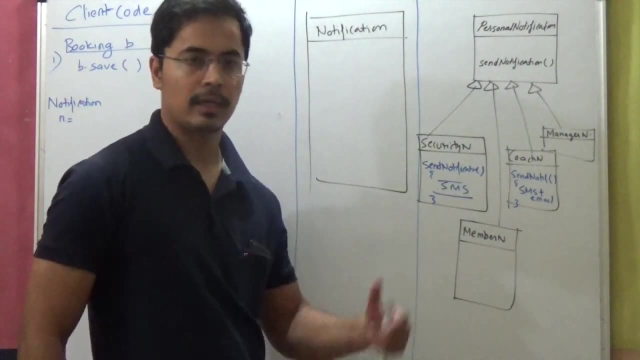 Of course, this itself is a design problem. We can't have duplication of SMS and email code in this classes, But we will solve it when we are doing the implementation of this Right, Because we don't have scope to discuss all that right now. 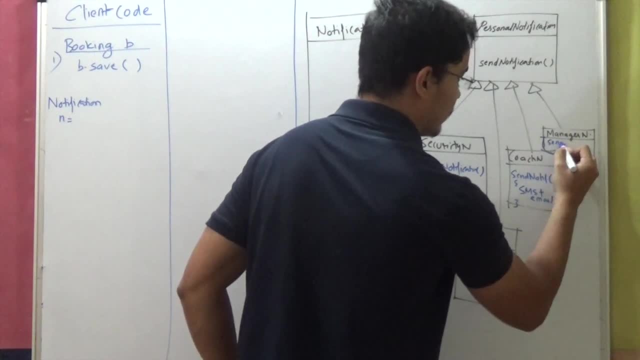 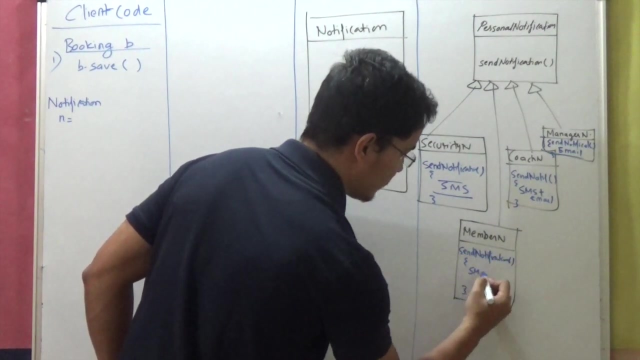 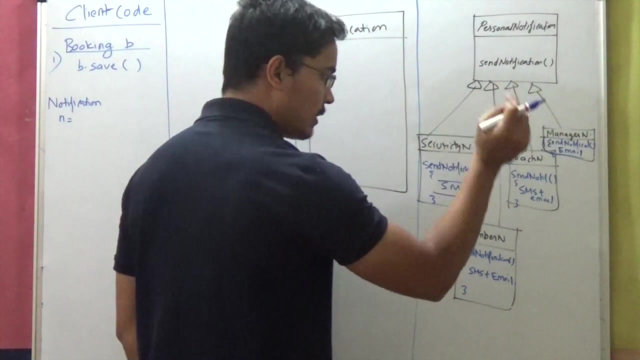 Manager in its send notification Notification implementation. It will only have email Right And member in its send notification will have SMS plus email. Now, So these are my concrete implementation of notifications: Security notification, Coach notification, Member notification And manager notification. 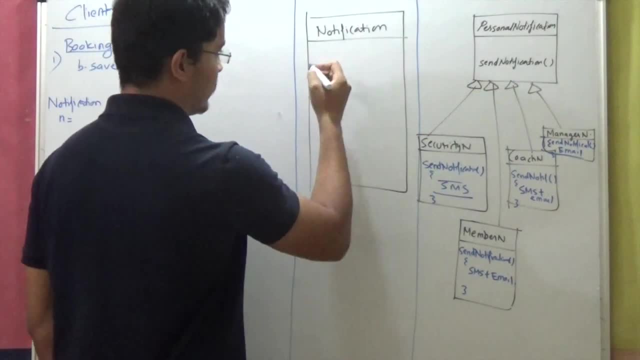 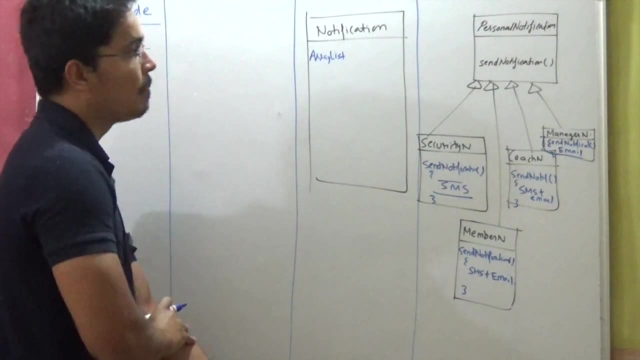 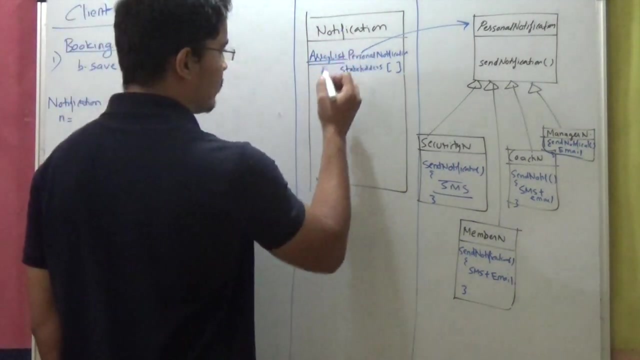 My notification class will be composition, So I will say Array list. It will be an array list of personal notifications, Right, I will denote it by array. You know, In class diagram. Now This will also require the context of the booking. 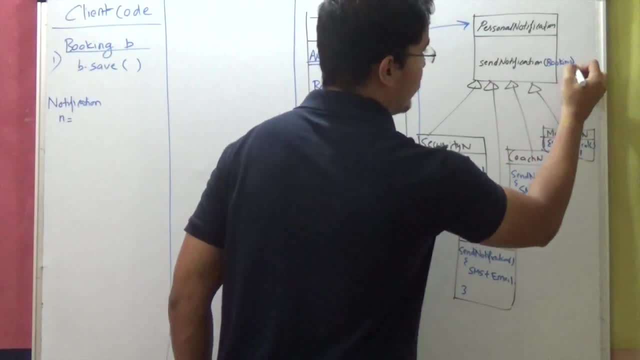 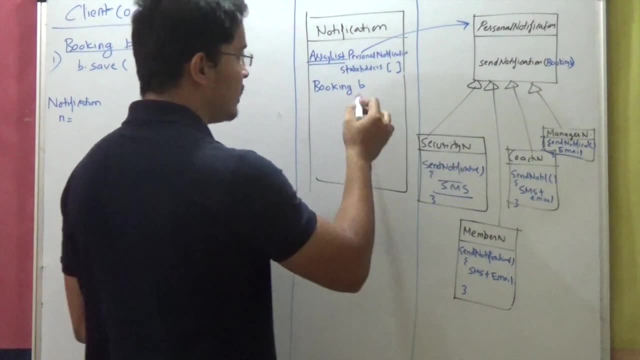 This booking context will also be used here. We need the booking context So because who has done booking At On what date, At what time, All these details can be obtained from the booking context. So All these classes will get the booking context from the parent class. 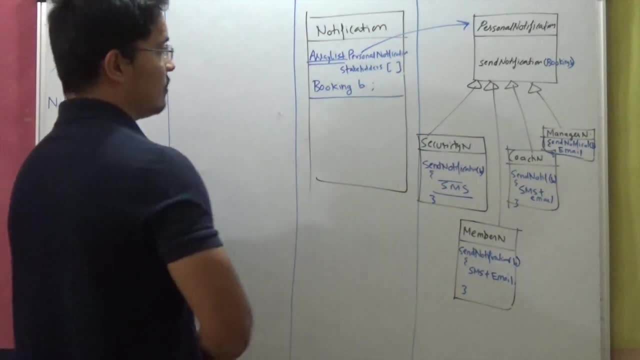 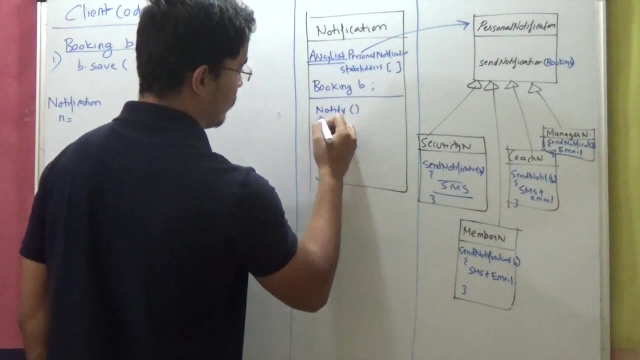 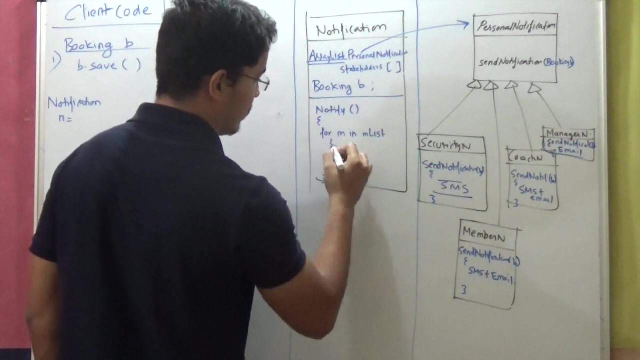 That booking context will be passed to the array list members. Further, We will have one notify method Here. The notify method will be very simple. For each element of this list, Let's call it as M list, Right, Right, We will say. 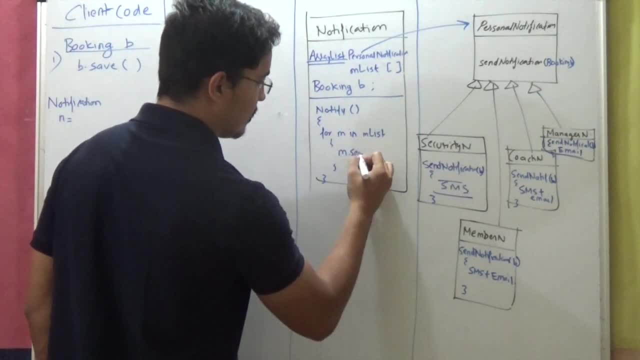 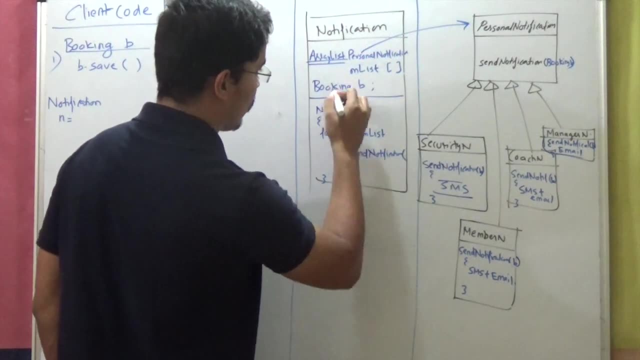 M Dot Send Notification. The Notification Right And I will pass the context of booking To that Right, So I will call. Invoke the send notification method of For each participant in this list, Which will be of base type. 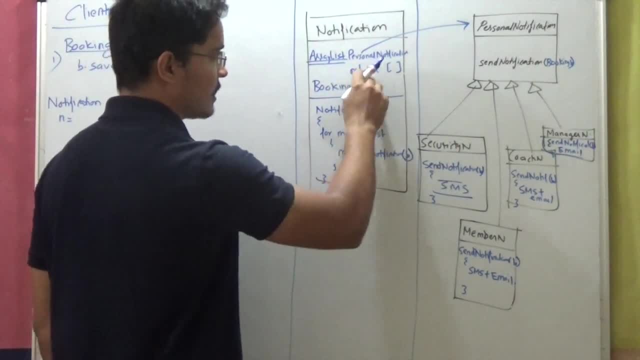 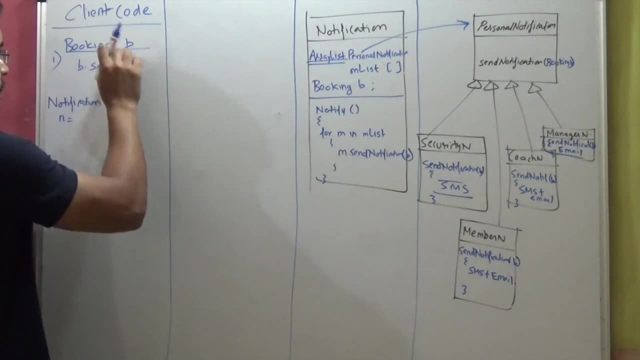 This Could be any of this Right Now, As we discussed in the beginning, Depending on the type of booking, Whether booking is a individual member booking Coaching session Or a Group booking by Lifetime members, Right So? 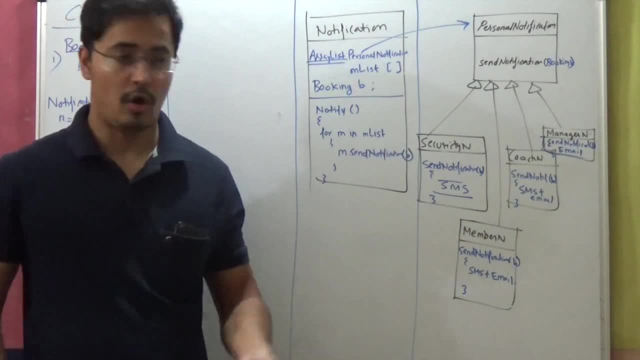 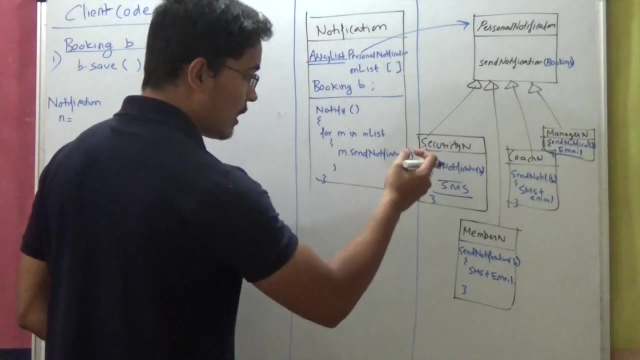 I will call. Invoke the send notification method of For each participant in this list, Which will be of base type. This Could be any of this Or a Group booking by Lifetime members. We will send notification To Some of them. 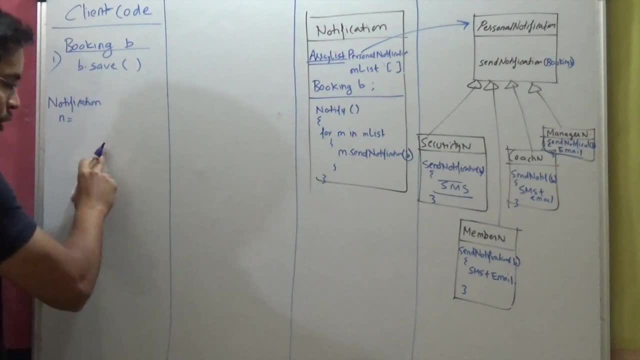 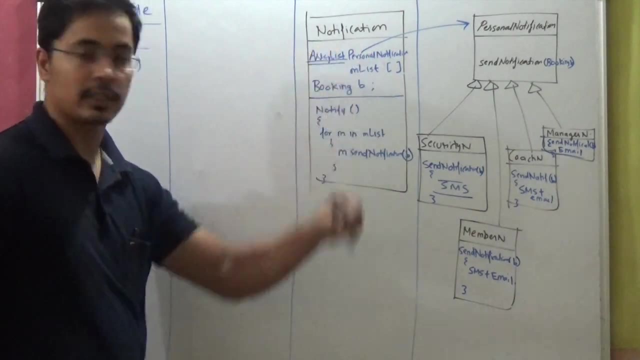 Or all of them Depends on the type of booking. So That code Of deciding Right How to build this notification. What will be the composition Of this notification class? Will it be consisting of Only security And member? 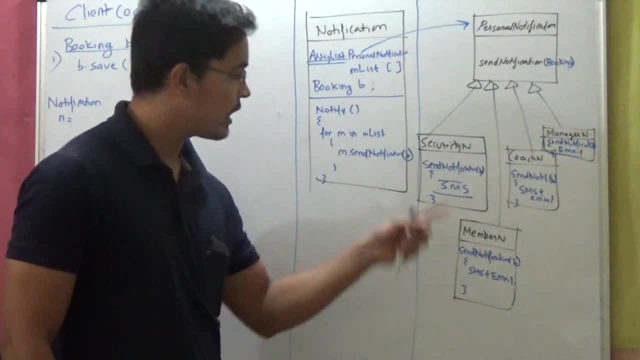 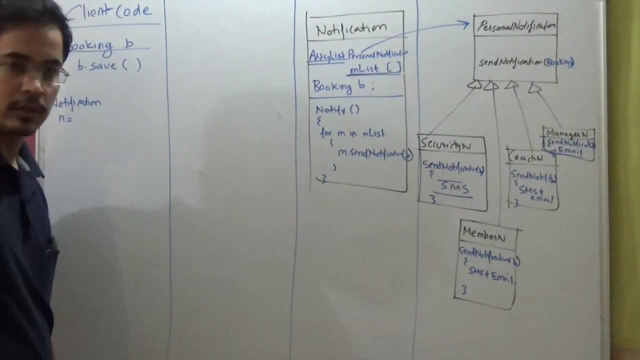 Or will it have Security Member And coach, Or will it have Security Member, Coach And manager? Depends on Type of booking. So If This, Then ArrayList Will have This And If not, 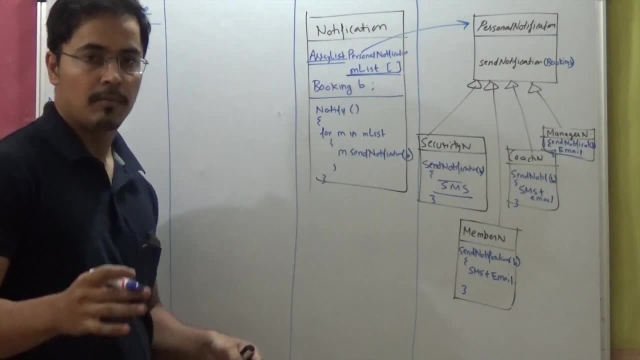 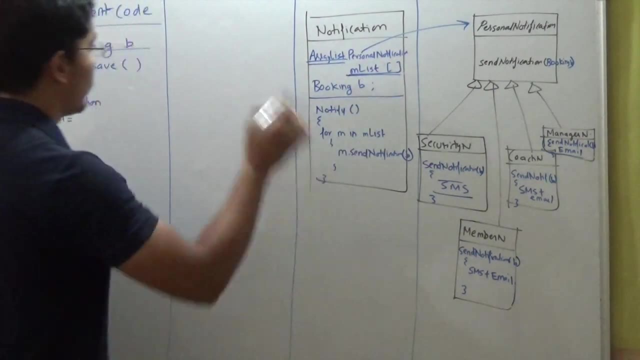 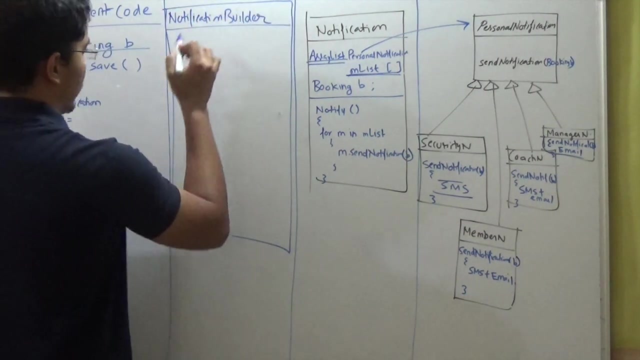 Then ArrayList Will have These. If not In other type, ArrayList Will have These. So Instead, Because We are using Builder Pattern, Will remove That Responsibility From Client And Notification. 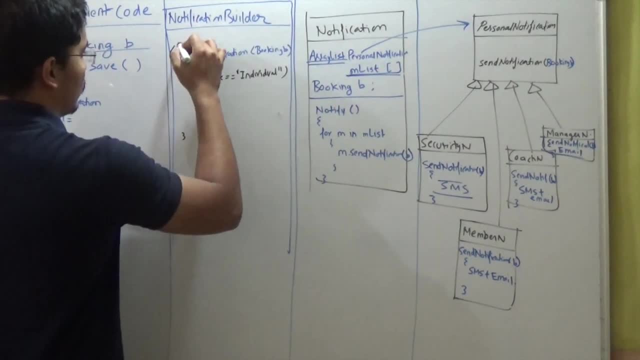 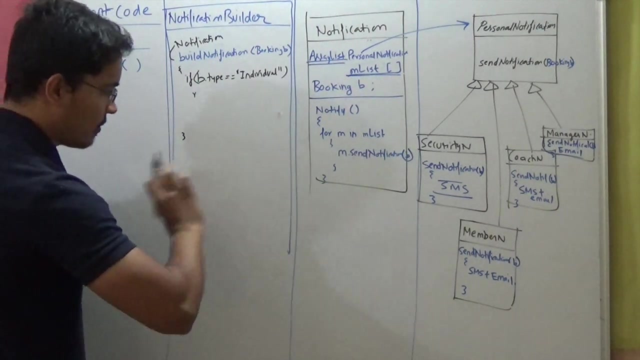 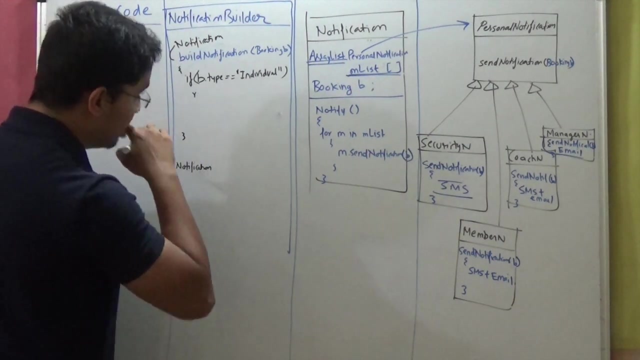 And It Will Require A Booking. So This Will Return Actually Notification, Because This Is Building Notification. The Return Type Of This Method Will Be Notification. 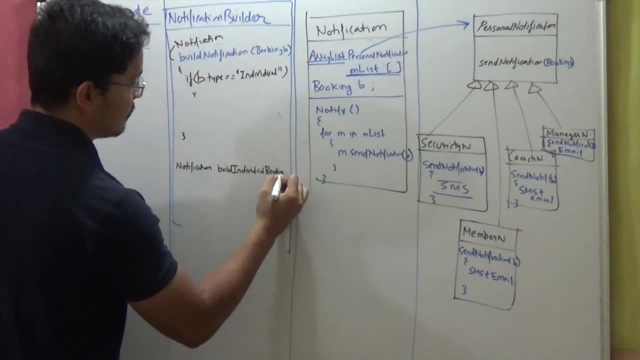 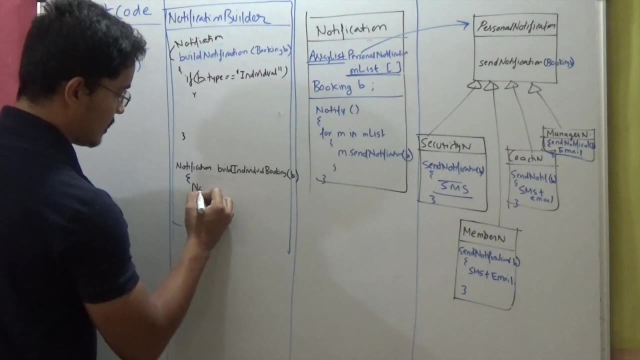 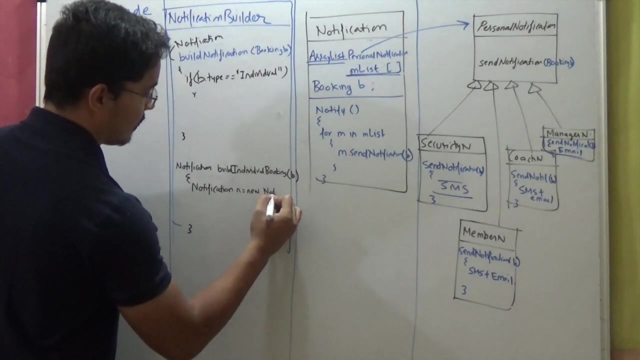 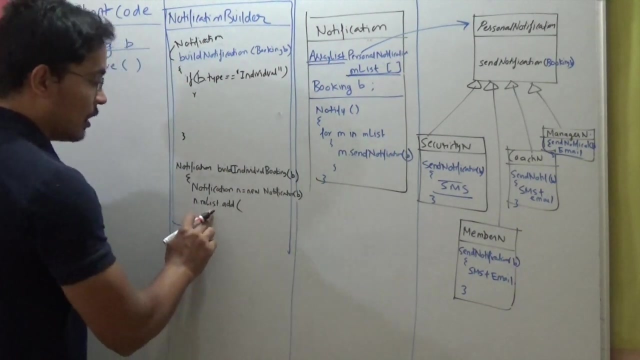 So Booking Notification, So It Will Also Have Booking Instance And Here Will Create One Notification. Let's Say Notification N Equal To New Notification, Because 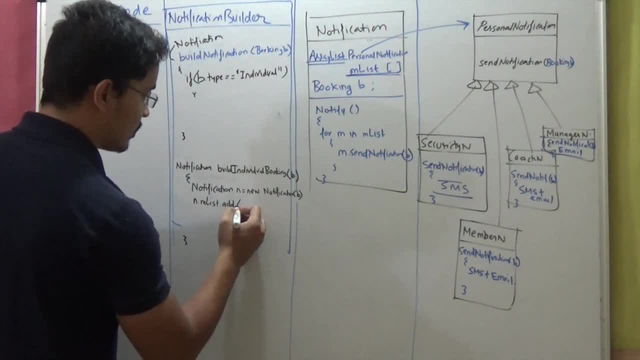 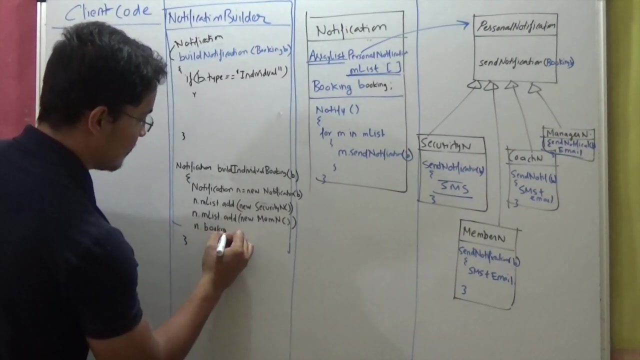 This Is A Individual Booking, So Will Create One New Security Notification Right And N M List Dot Add New Member Notification N Booking Equal To 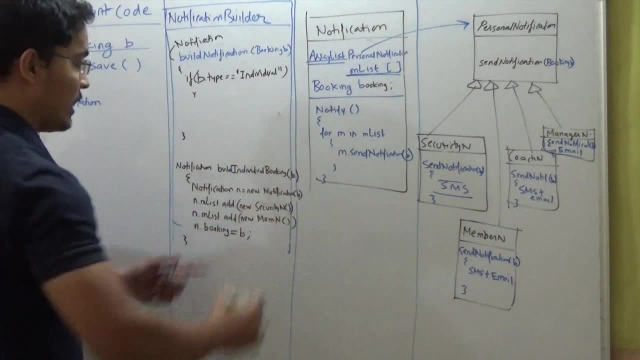 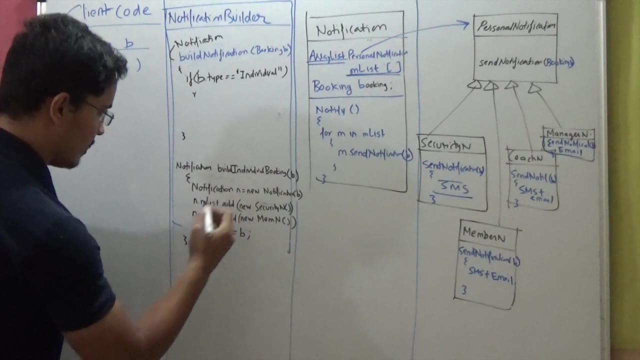 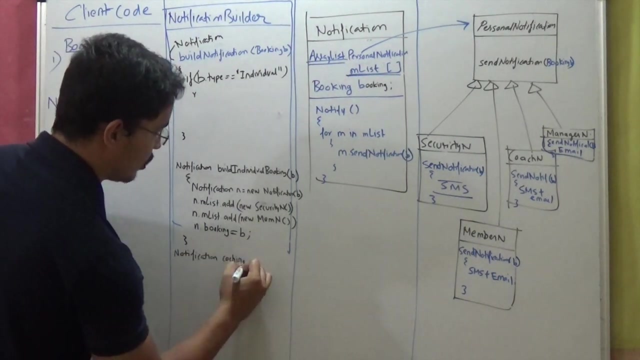 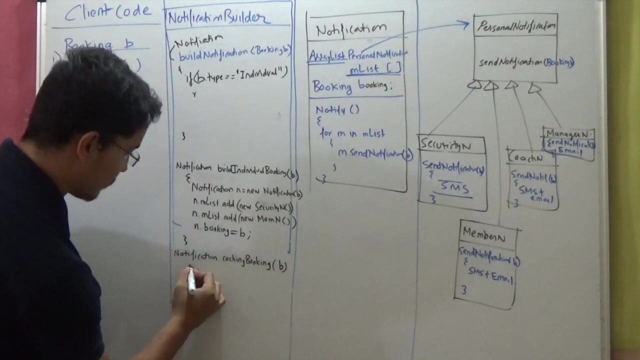 Whatever Booking I Have Received. So This Is Coaching Session. So Similarly Will Write Another Helper Method Here. Let's Say It Will Return Notification Coaching. 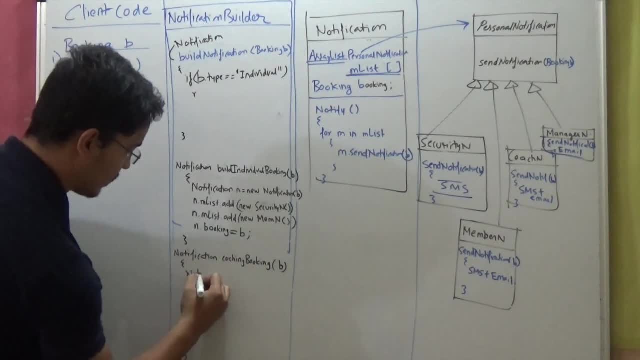 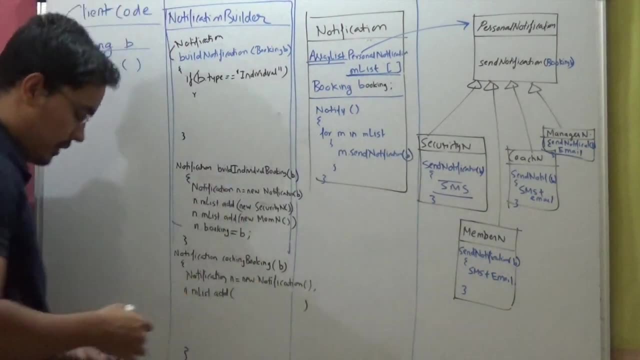 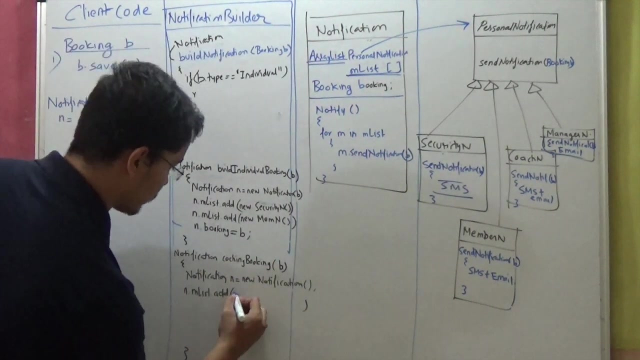 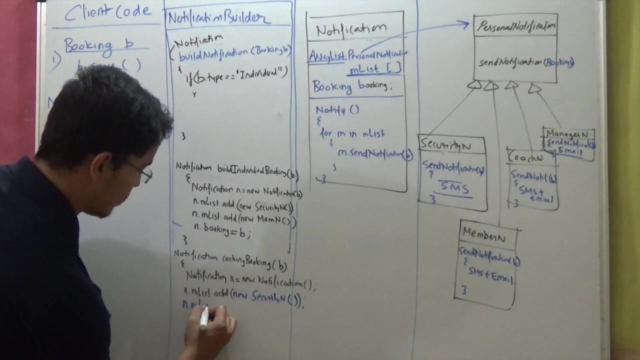 Booking Right. This Will Also Require A Booking Context That Will Get. We'll Have To Send The Notification To Security Person, Member And Coach. So 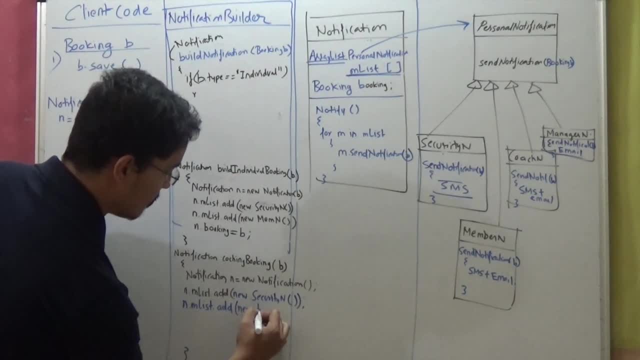 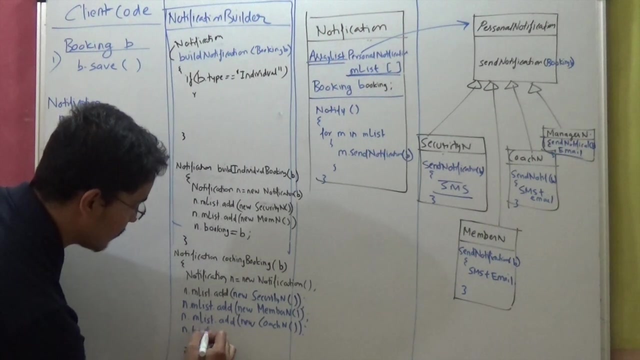 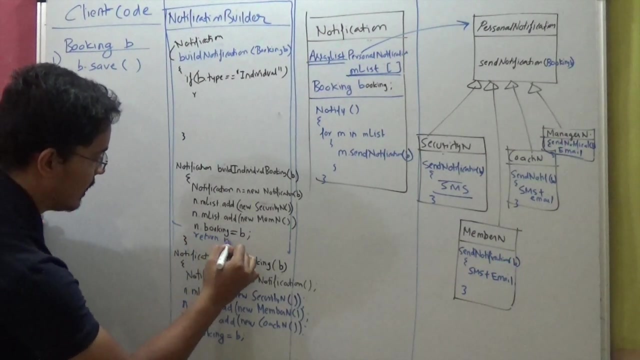 In This Case We'll Say New Security Notification. Then We'll Say N M List Dot, Add In Dot. Booking Equal To B Right And We'll 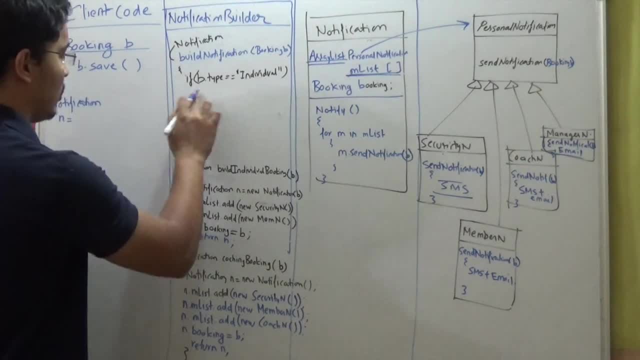 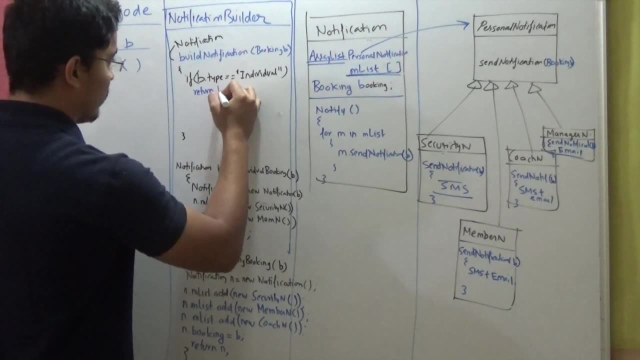 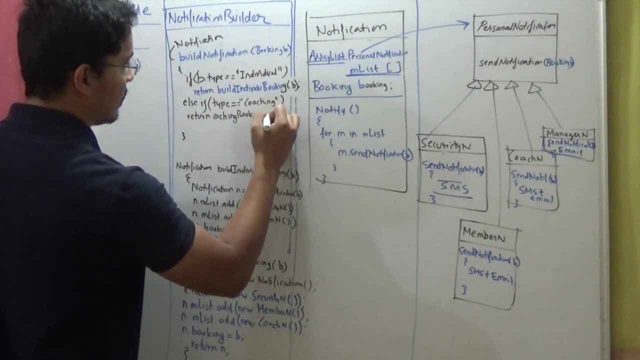 Obviously Say Return N And Return N. So If Booking Type Is Individual, We'll Call This Method. We'll Say Return Notification: Coaching Booking Notification. I. 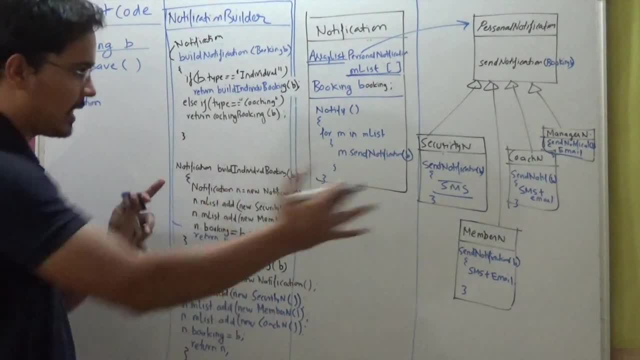 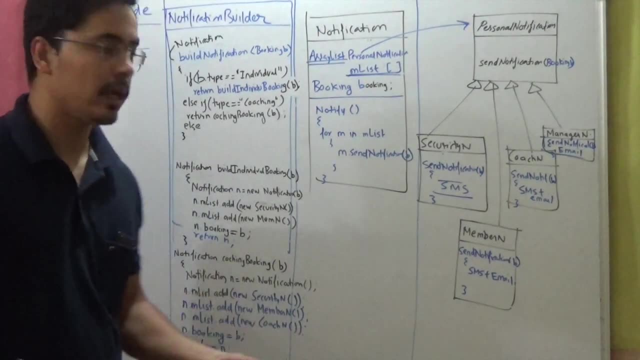 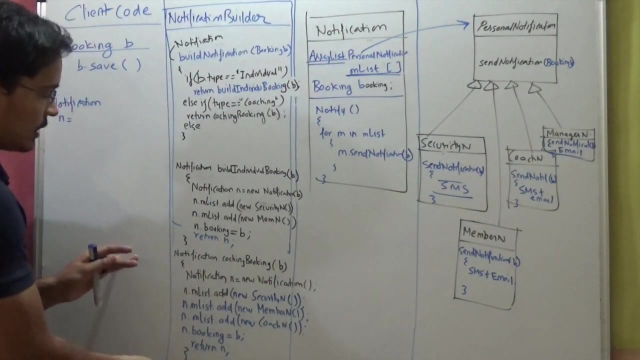 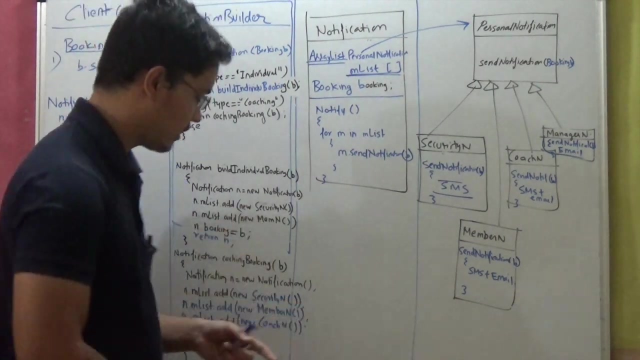 Should Have Changed The Name. I Know That Again, I'm Pressed For The Space Else, We Also Have To Write. One More Method, Remember We. 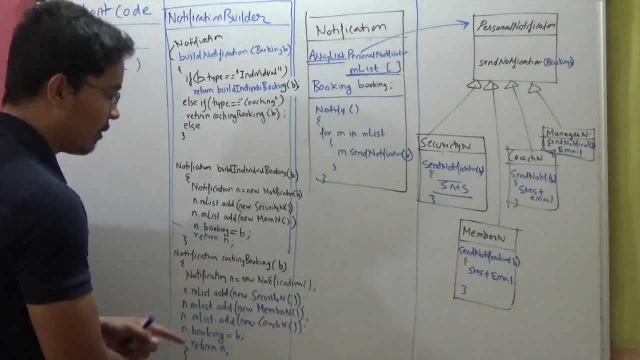 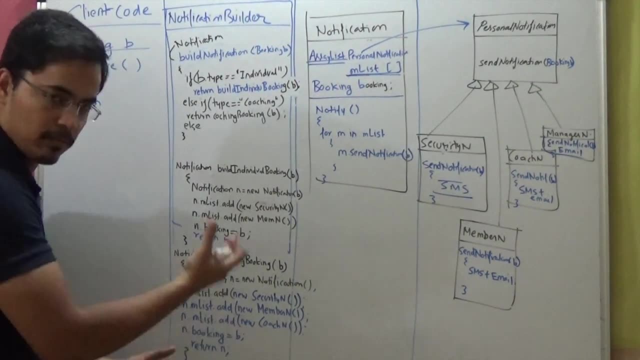 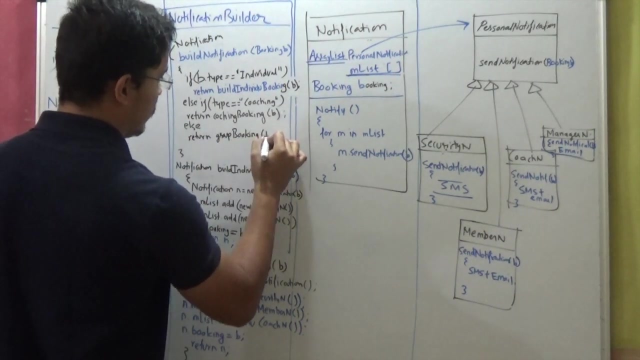 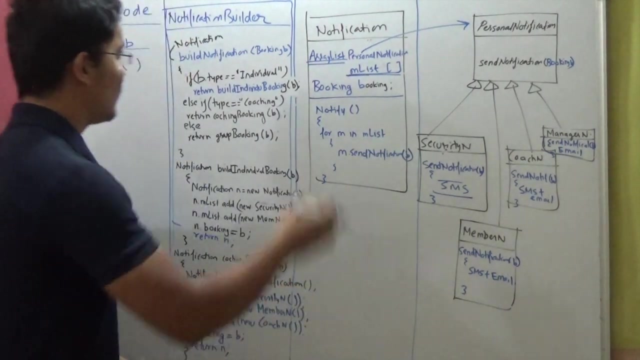 Have Notification Object M List. That Is A List Of Type Personal Notification. It Will Add One Instance Each Of Security Member, Coach And Manager And. 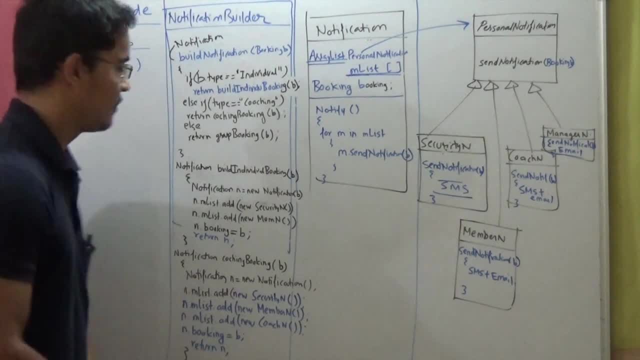 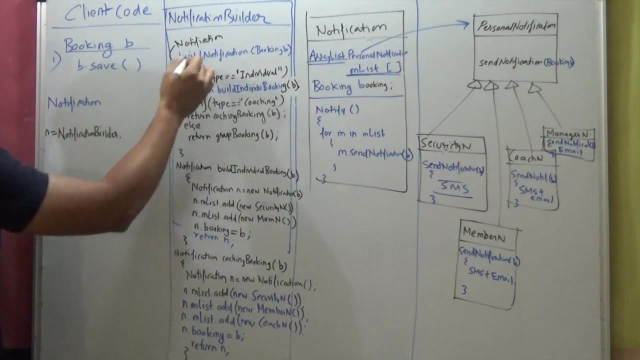 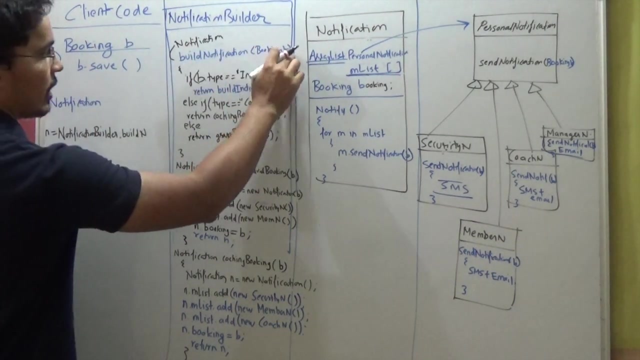 We'll Build. We Have To Do Almost Nothing. We'll Say Notification N, Notification N A New Object Equal To Notification Builder Dot. This Is Static. 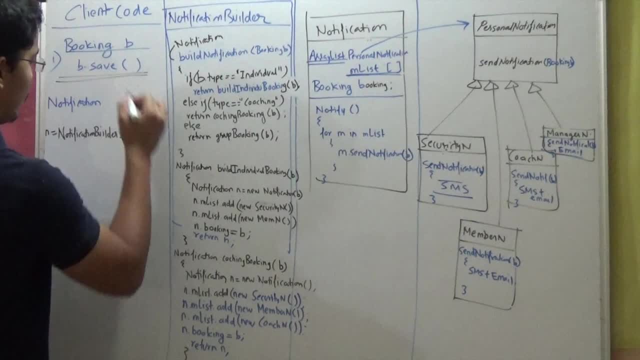 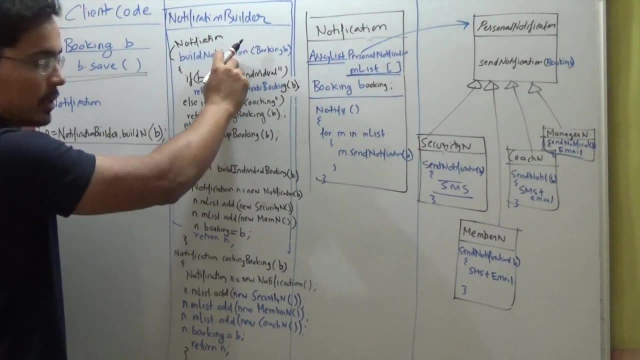 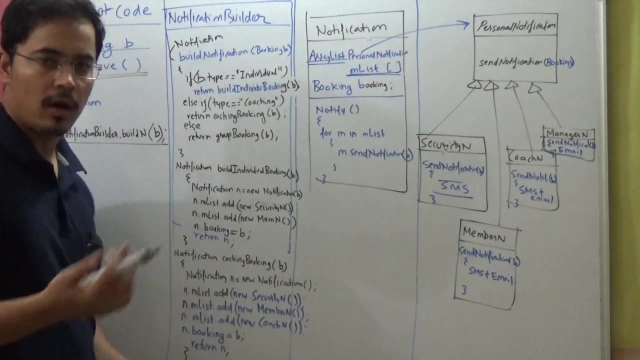 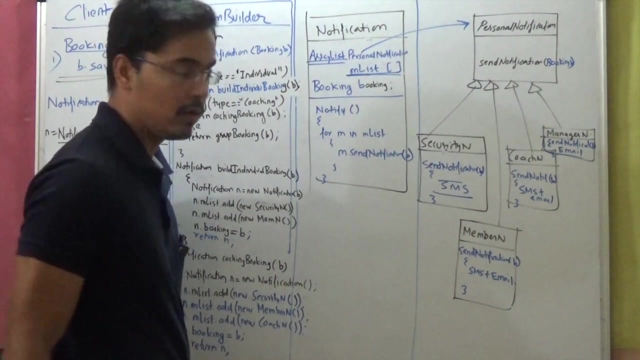 Method Right. So Return Type Is This Notification: Builder Dot Build Notification Method Will Take Into Consideration What Kind Of Booking It Is, Whether It's 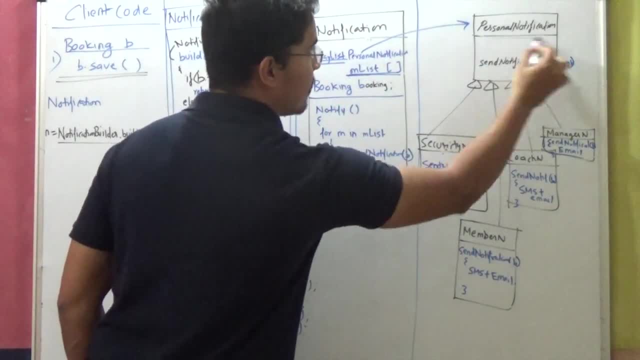 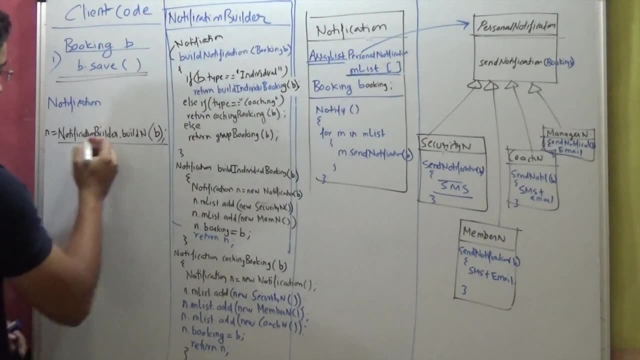 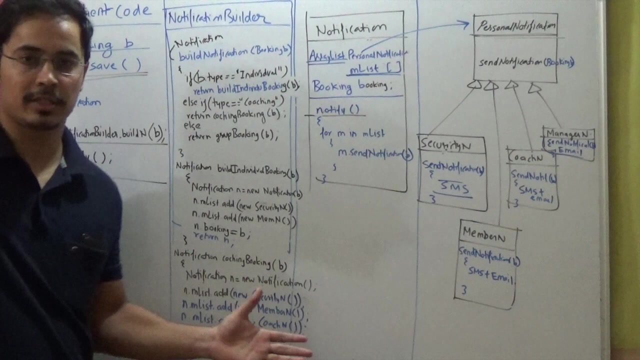 Individual Coaching Or Group Booking, Based On Which It Will Eventually, This Method Will Return Here. So Once You Get This, All You Got To Do. 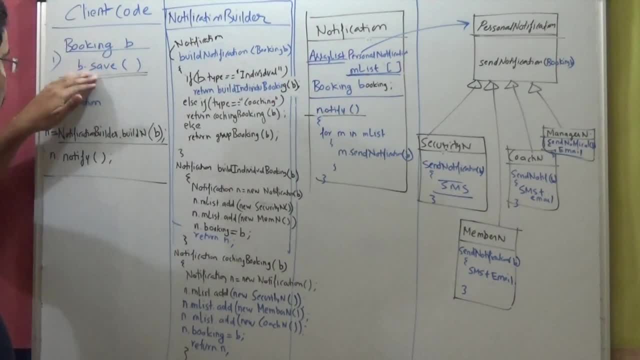 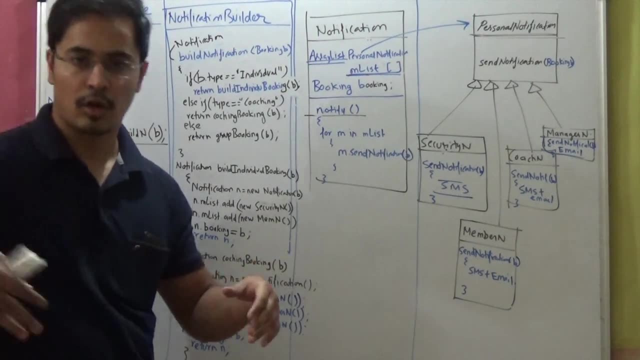 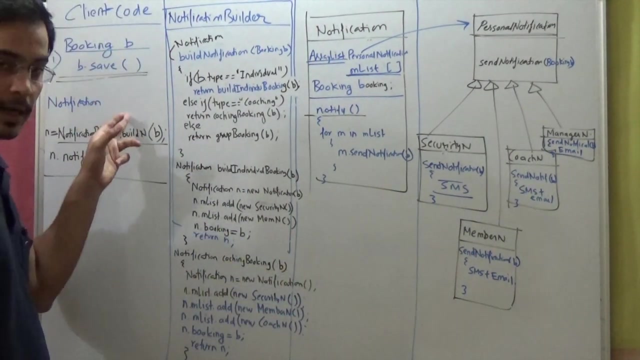 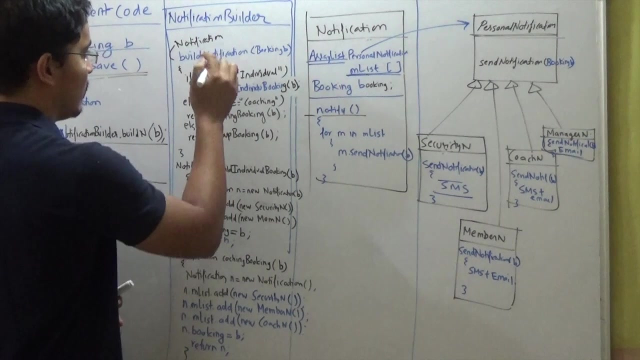 Is You Have To Say N Dot Notify, That's It. So Look At The Notifications Regarding That Booking. So Here In My Client Code I'm 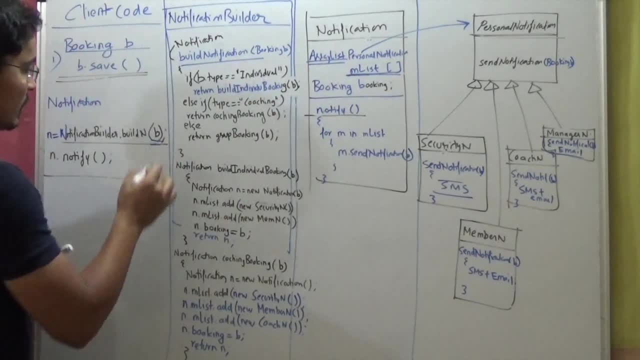 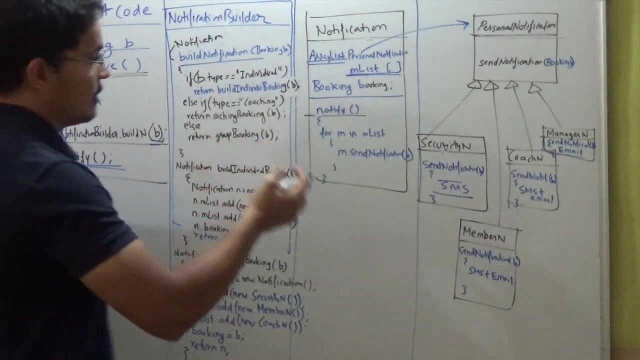 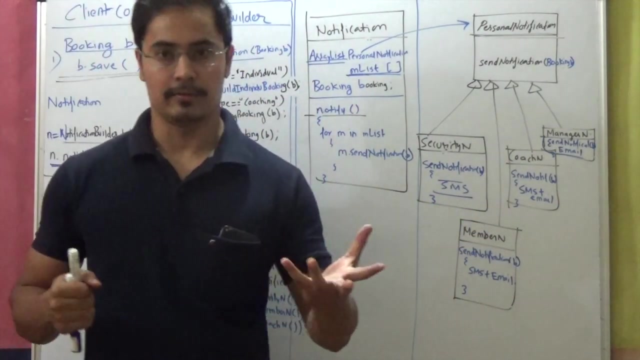 Just Saying Notification N Equal To. I'm Calling This Builder Class Static Method, Build Notification, And I'll So Look At This Complex Logic That We 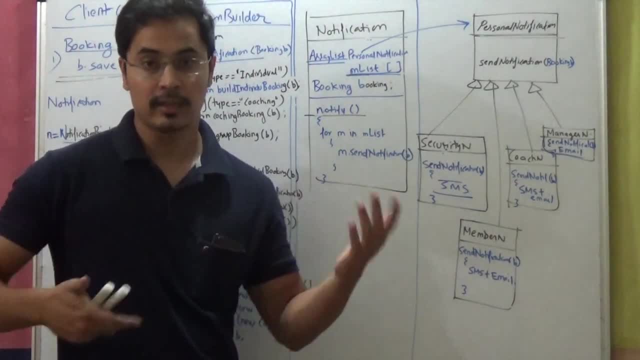 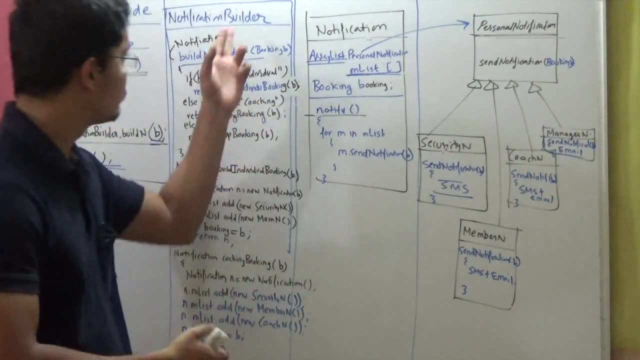 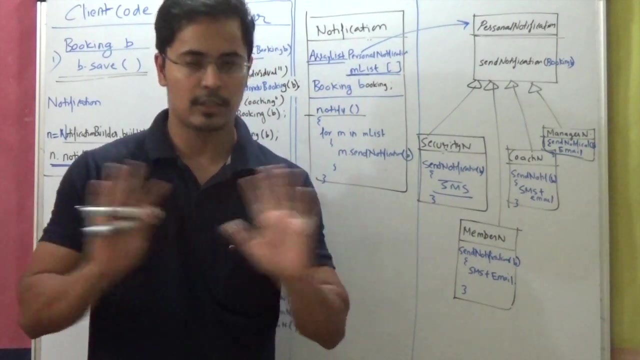 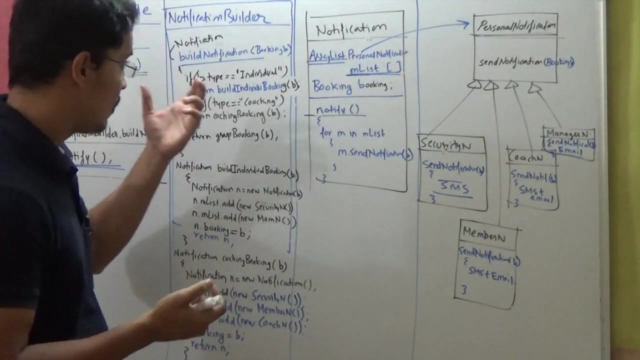 Are Hidden. We Have Abstracted From The Client. It Has Just Taken Care Of Saving Or Creating The Booking And Once We Are Taking The,